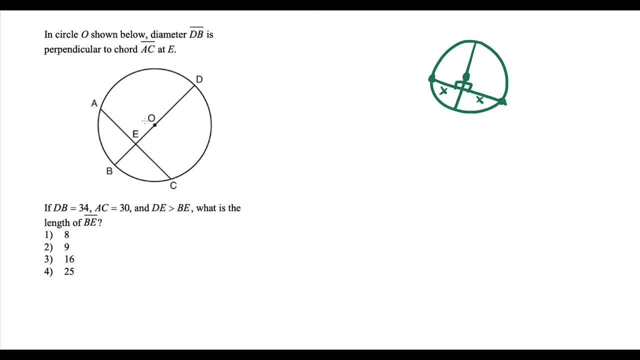 is going to cut the chord in half, So each of those segments would be the same. So notice here: diameter DB is perpendicular to chord AC. So that means that this diameter is going to cut this chord in half from here to here. So if the whole thing is 30, that means each. 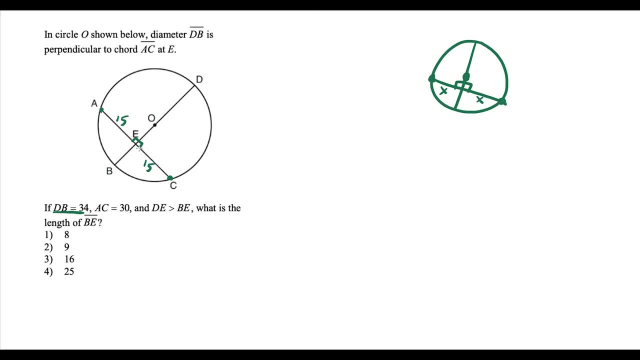 piece is going to be 15.. And what we could use next is the entire diameter is 34.. And the radius, just know the radius of a circle is half the length of the diameter. So if the whole diameter is 34 units, if we take half of that, that tells us any radius that. 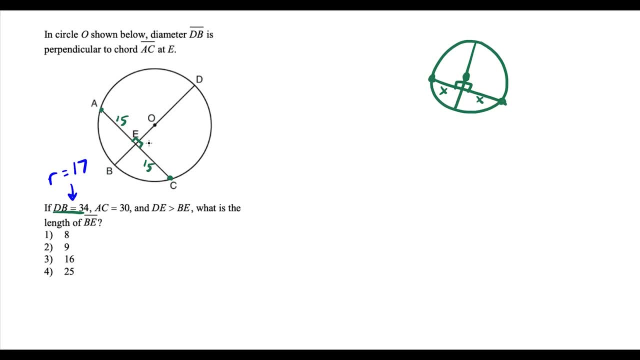 we construct is going to be 17 units long. So now the goal here is to find the length of BE. So we want to find the length of this segment here, Okay, Okay. So to do that, what we're going to do is we're going to construct a radius And we 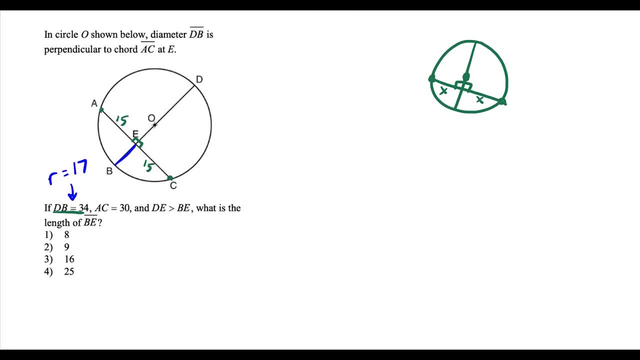 could construct the radius over here. So let's draw that a little bit nicer. So, OC, And once again, the radius is 17.. So no matter where I draw this radius in, it's going to be 17.. But notice, now we have a right triangle. So we're missing this side, OE, but we know this. 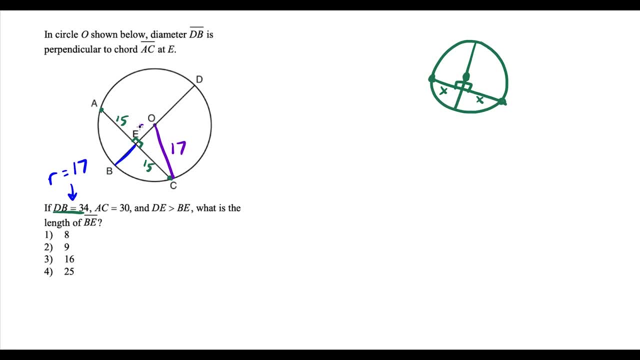 side is 15 and this is 17. So if you know your Pythagorean triples, it should jump out at you that OE is equal to 8 units. So we could say OE is equal to 8 units And we could do that. But if you want to fact check this, you could just do 8 squared plus 15 squared. 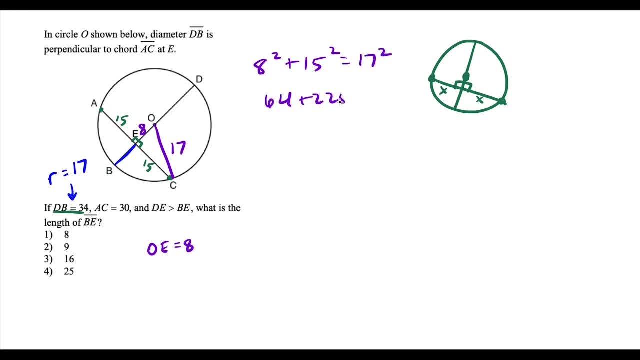 equals 17 squared and 64 plus 225 is definitely equal to 289.. So this is definitely going to check out. But now, once again, we said all the radii are going to be 17 units long. So OB is another radius and OB from here to here is equal to OE plus EB. So once again, the 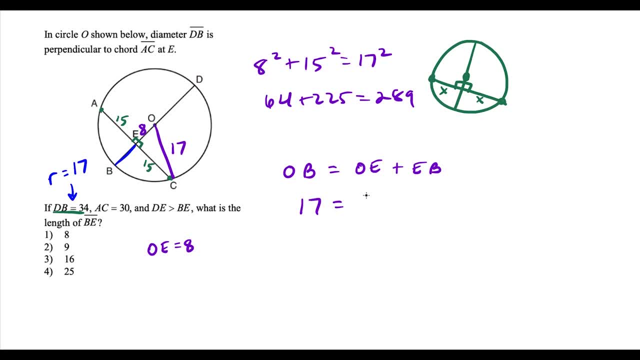 radius OB is also 17 units long. Okay, So this is going to be 8 units long And if we do plus EB, this tells us that EB, if we subtract 8 on both sides, is going to be equal to 9 units. So this is going to be choice. 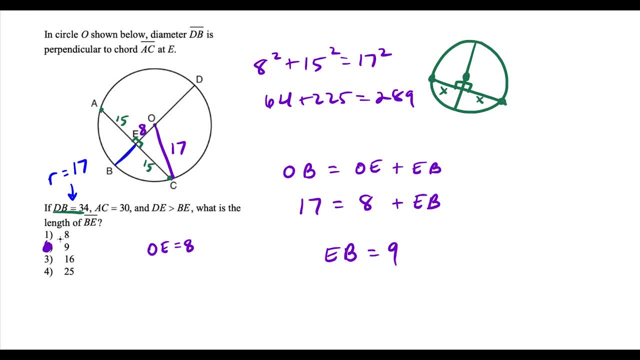 two, Okay. Well, this is going to conclude this video. If this video was helpful, please like and subscribe. It really helps me grow the channel And if you have any requests, just leave the topics you want me to cover in the comment section below. And thanks for watching.